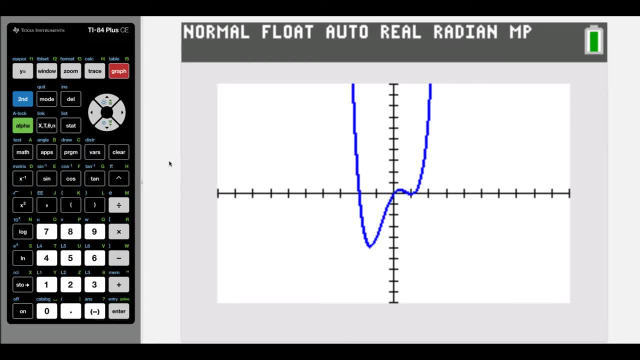 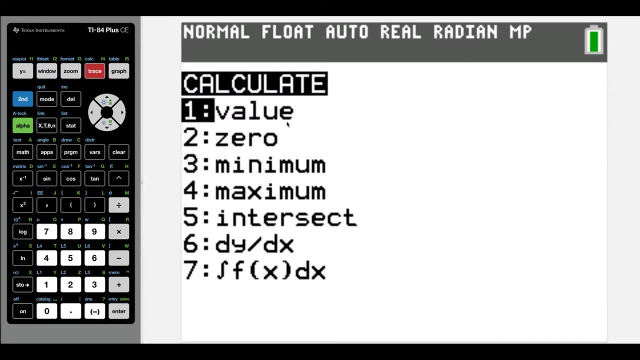 Now we can actually use our calculator to help us find a pretty exact value as to where those maximum and minimums are happening. So what we're going to do is we're going to hit second and then our trace button, And if we look in our options there, 3 and 4 give us an option for finding a minimum and a maximum value. 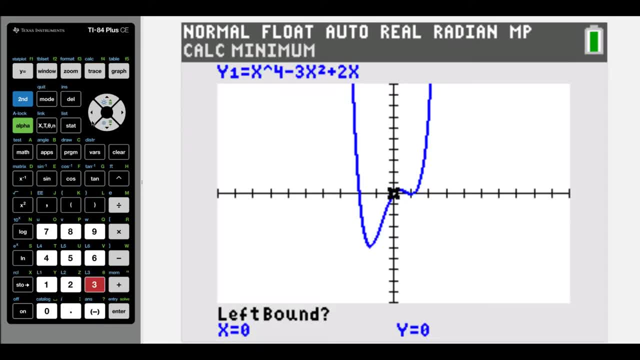 So I'm going to start with number 3.. I'm going to start with a minimum. Now, what it wants is a, a left-bound point. So if I'm focusing on this minimum at the bottom of this bigger valley over here, 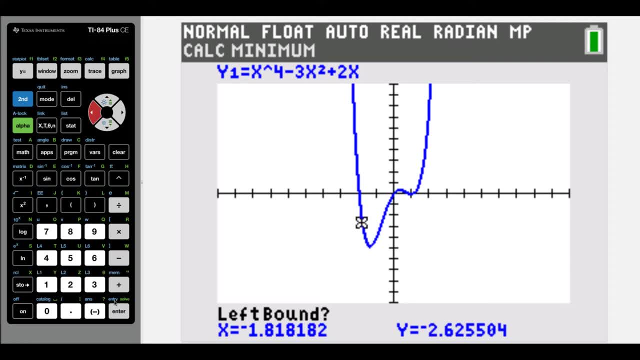 left-bound means I want to start on the left-hand side of that valley And I'm going to hit enter And then a right-bound point. we want to arrow over to the right, past that valley, And what it's going to do is it's going to look between these two lines that it puts on my graph for the lowest point. 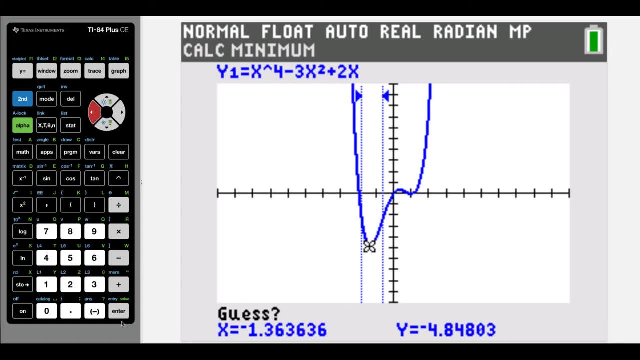 Now we can take a guess, but it's not 100% necessary. So maybe our minimum is about right there. I'll hit enter And it's going to tell me where my minimum value is. So this ordered pair, this x and y value, is the minimum of that graph. 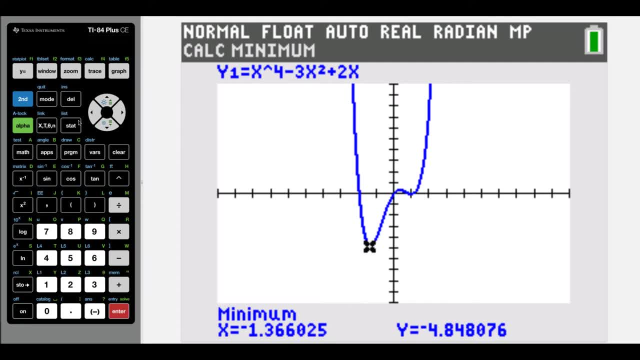 Now there is also another minimum happening up here. So we can find that one by doing the same thing, So going second trace and picking option number 3, minimum again. So now we want to arrow over by that other minimum. 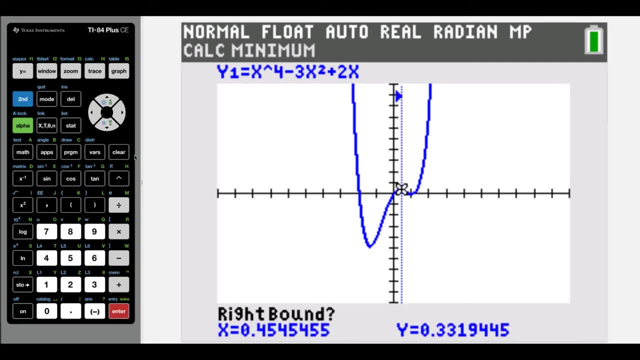 And again we want a left-bound point. So I'm going to hit left a couple times, Hit enter And I'm going to go to the right past that value And hit enter. We can take a guess, but we don't have to. 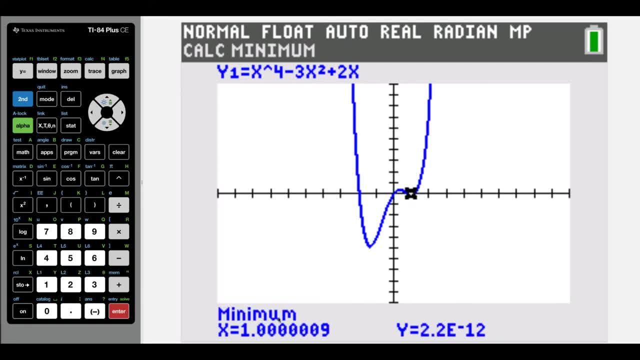 We can just hit enter one more time. So there's our relative minimum there. Now, as you look at your y value, you're going to see some stuff that looks like scientific notation. So what we've got is 2.2 times 10 to the negative 12th. 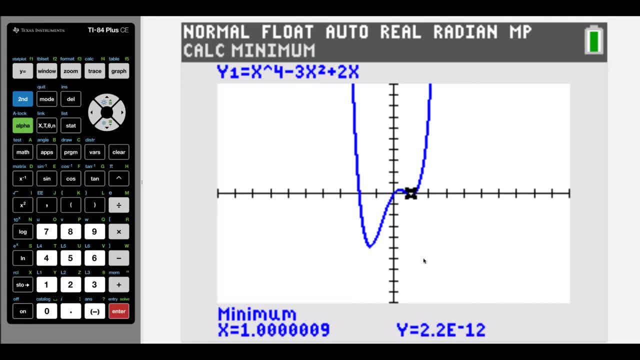 What we need to be able to recognize is that times 10 to the negative 12th really means a left slide with our decimal point 12 spaces. So we'd get a decimal with a baseline And we'd get a big long string of zeros leading it off.